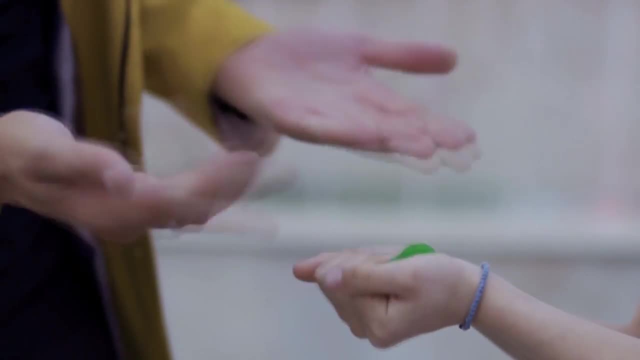 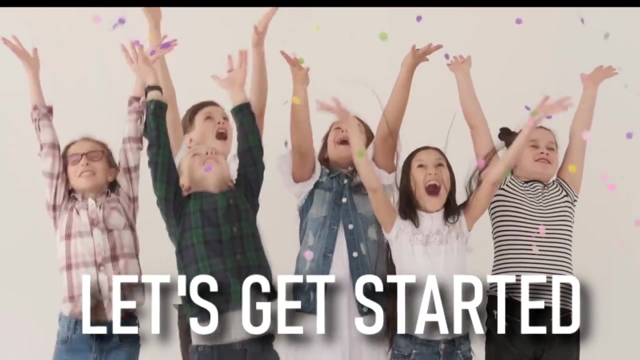 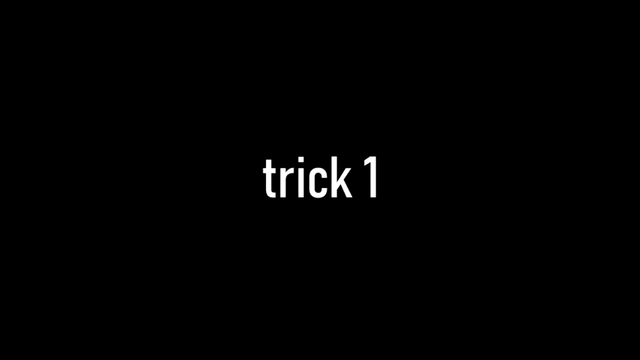 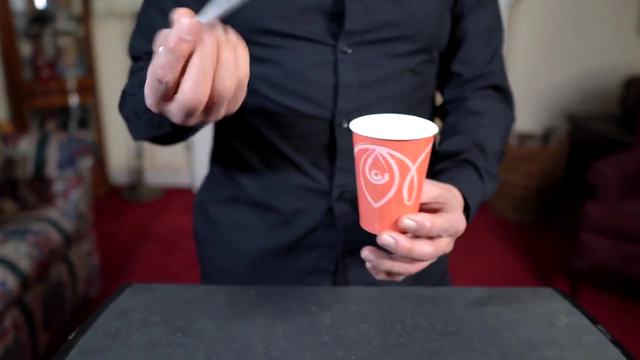 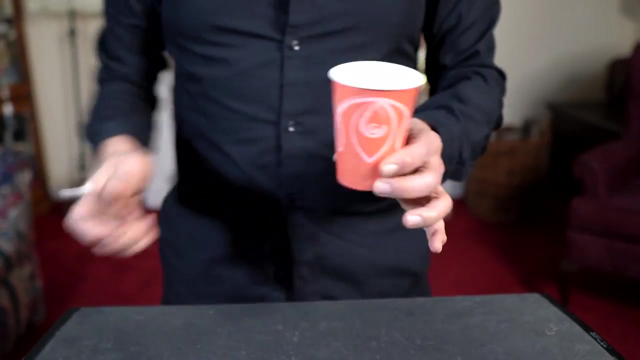 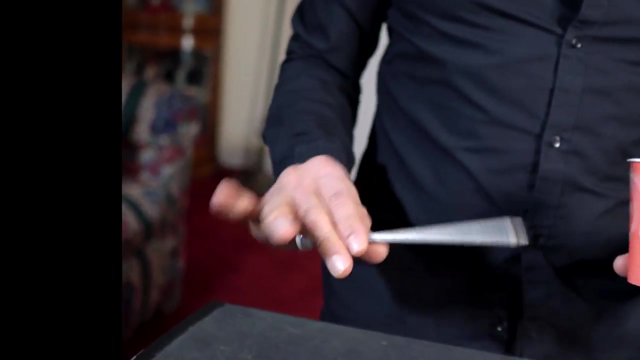 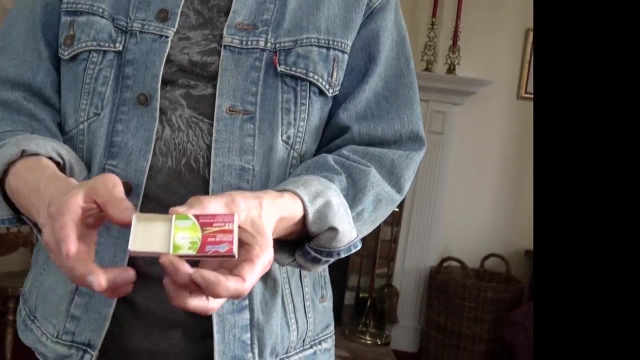 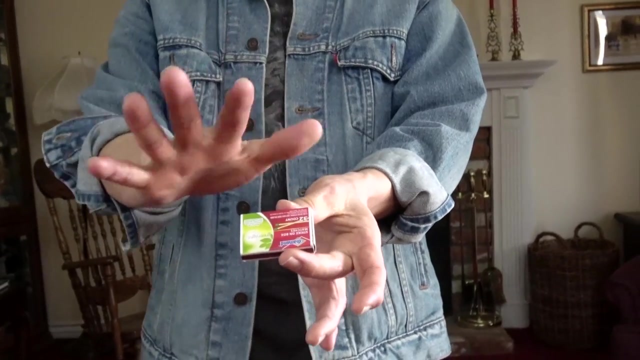 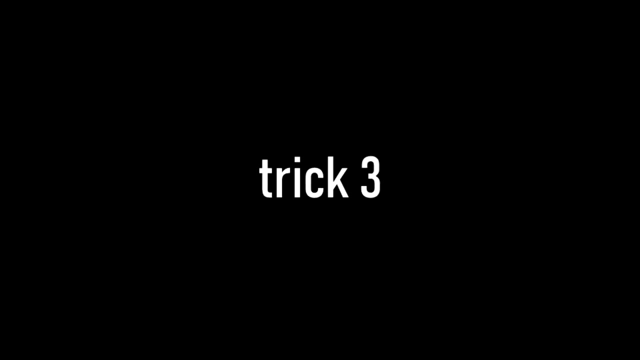 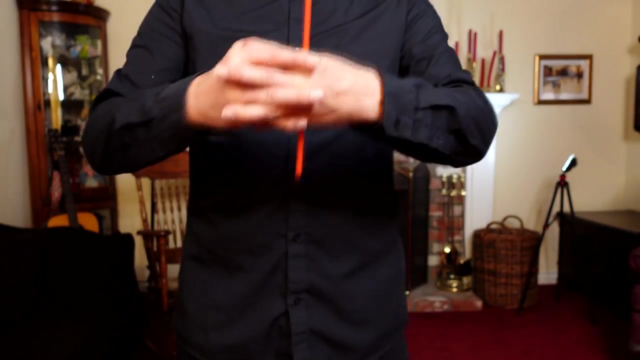 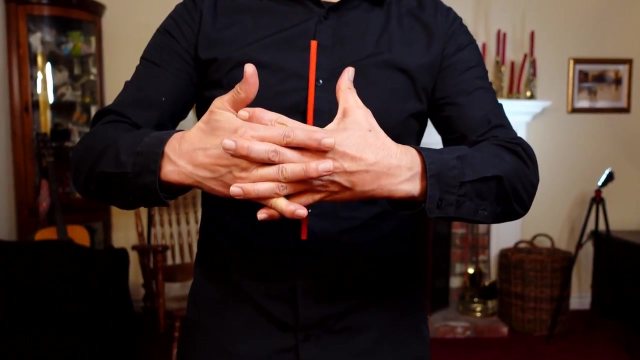 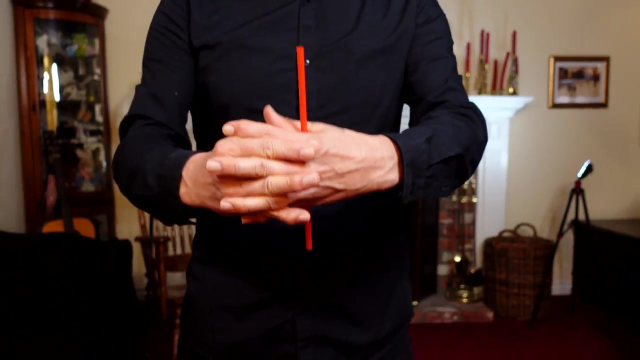 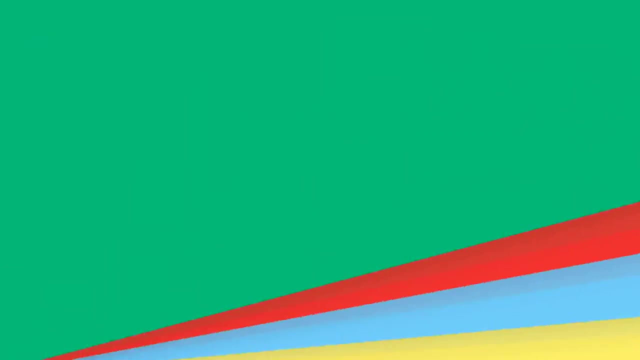 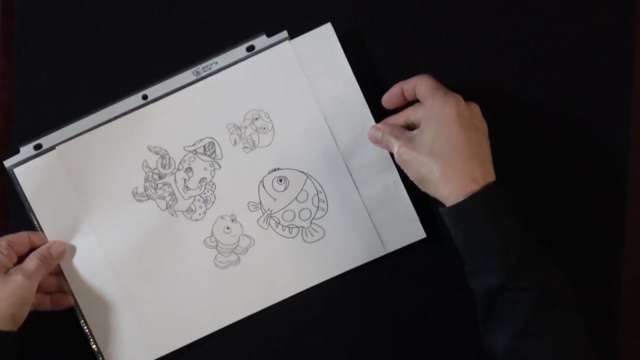 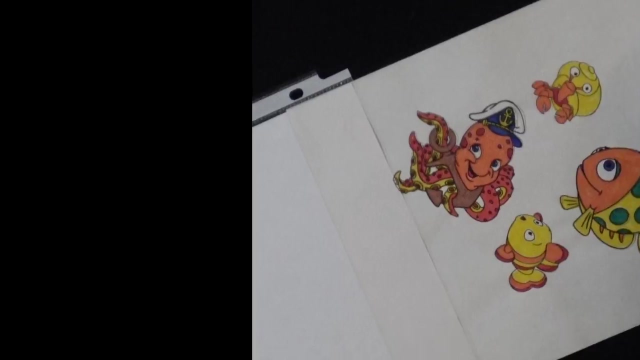 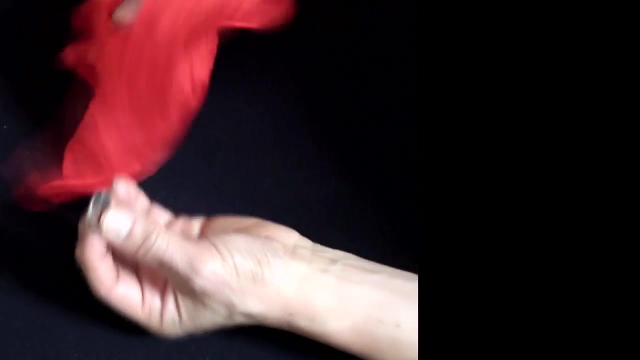 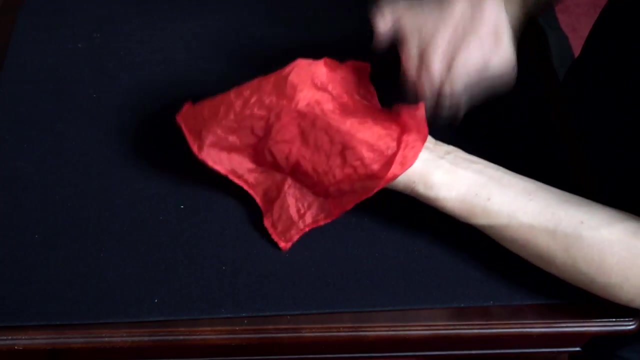 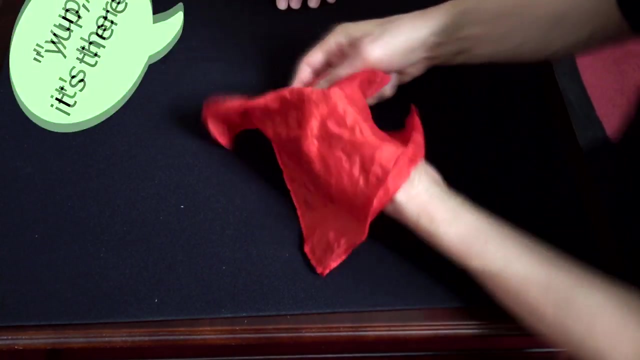 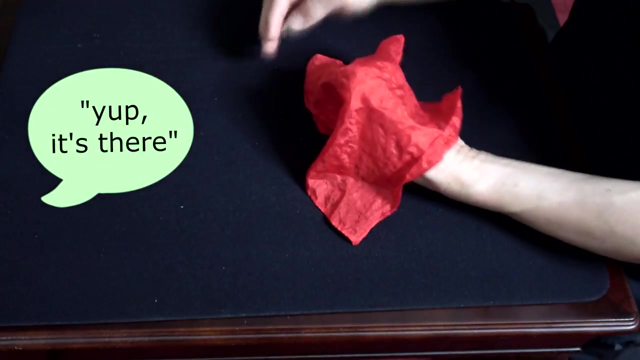 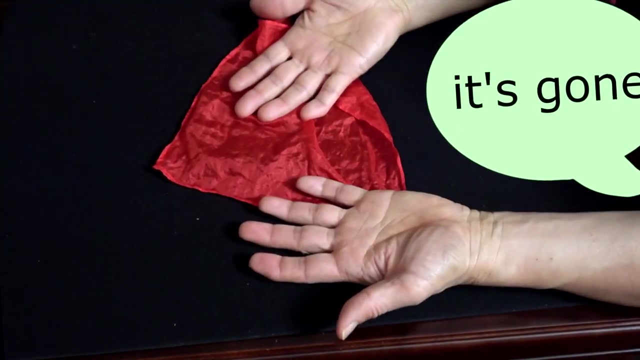 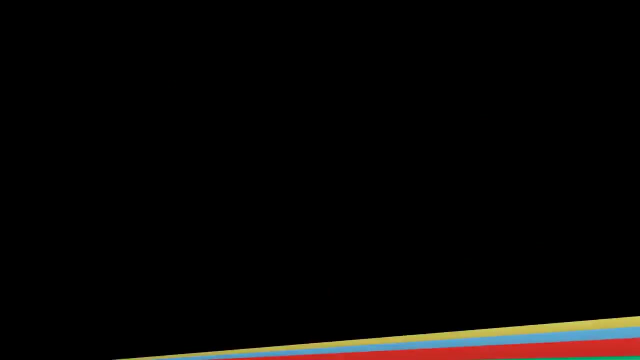 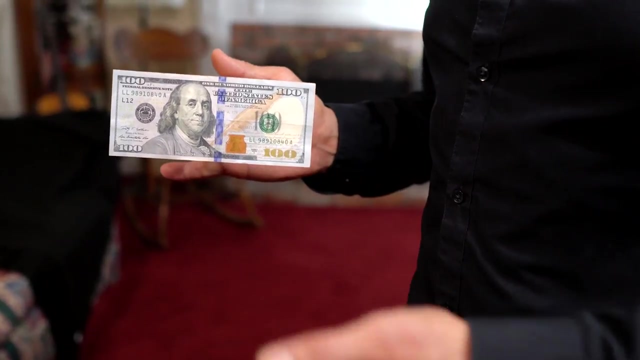 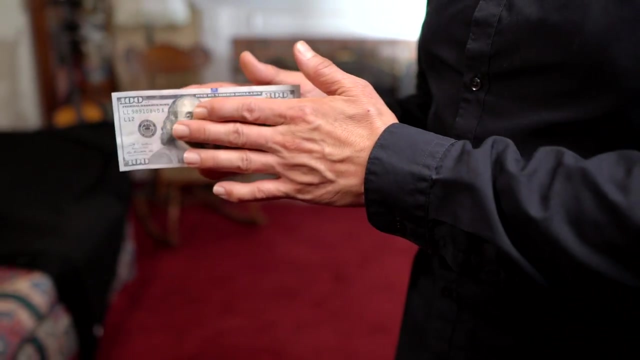 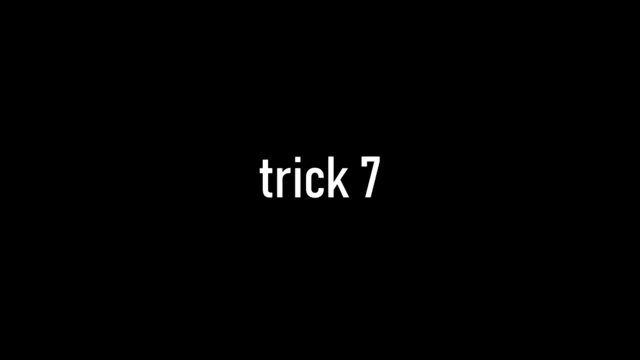 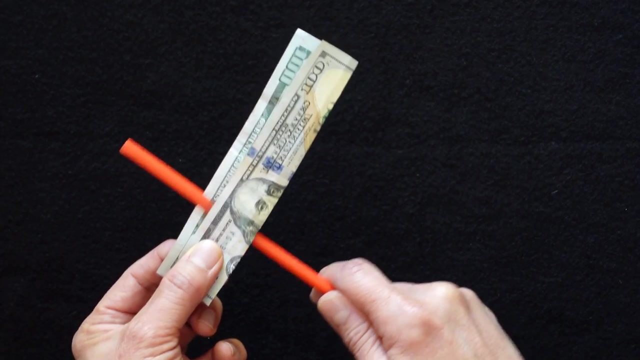 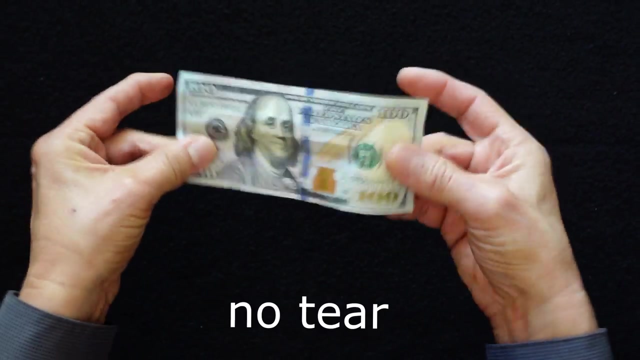 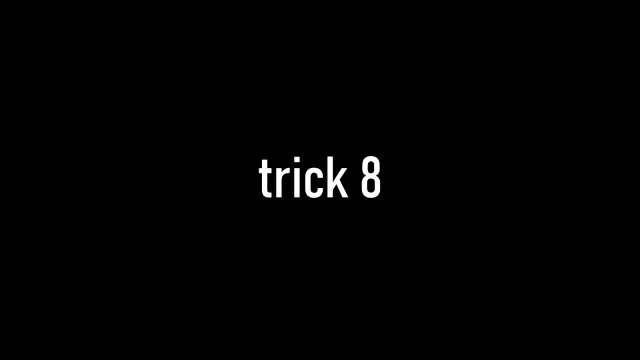 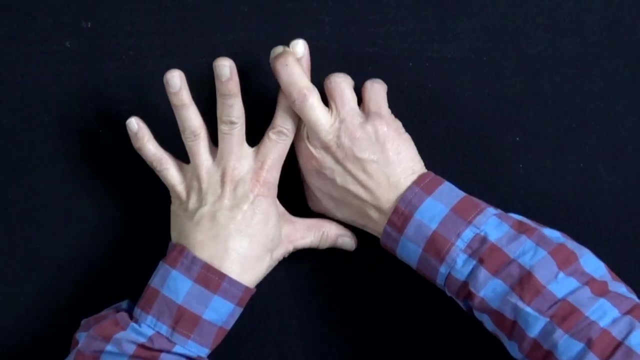 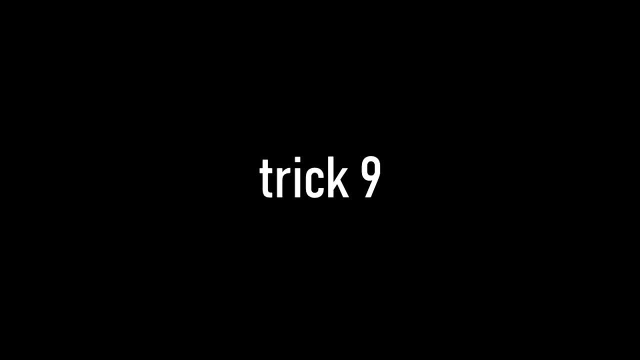 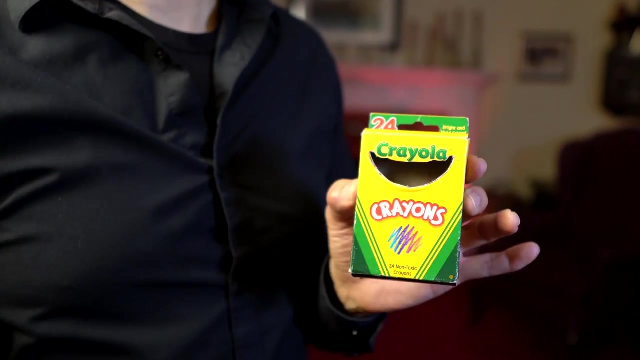 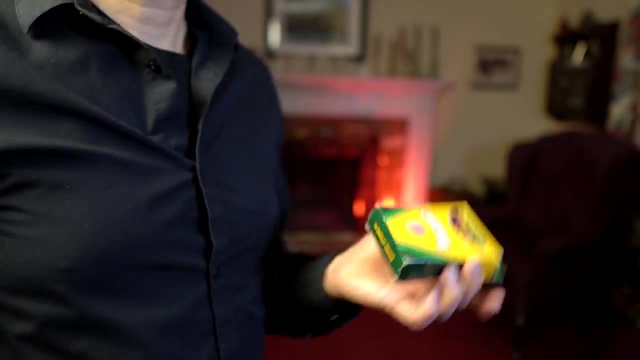 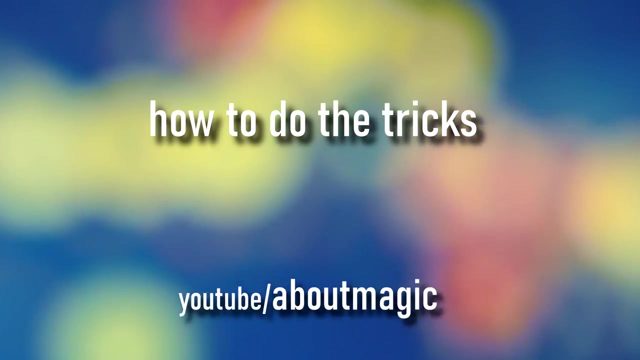 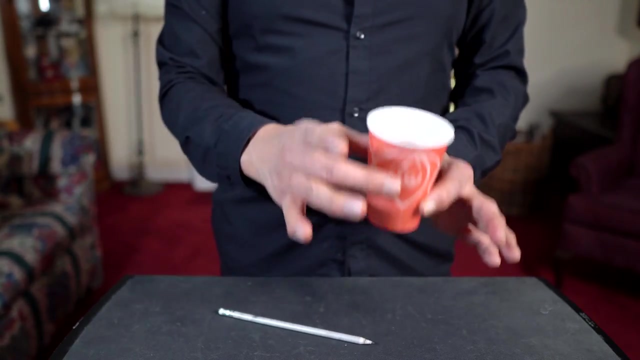 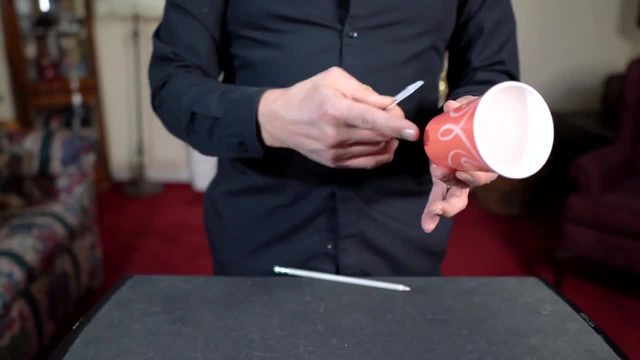 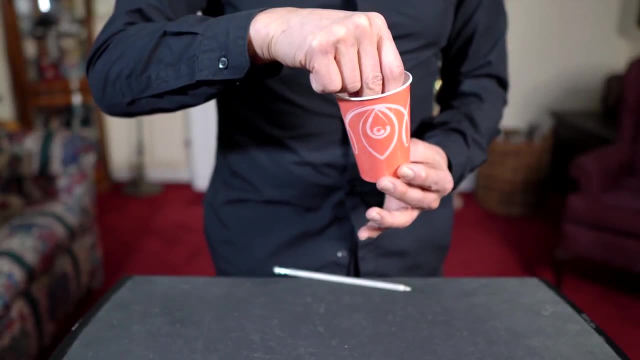 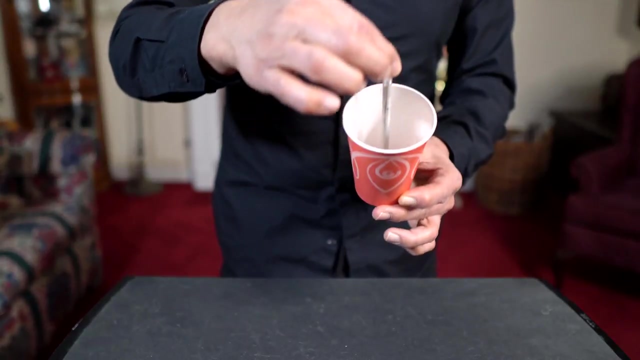 Actually, you need two cups because you need to cut the bottom out of a second cup And, as you can see here, there's a hole at the bottom. So the way this starts out is you have this flap Leaning against the side there, you take your pencil and you push it through the hole. 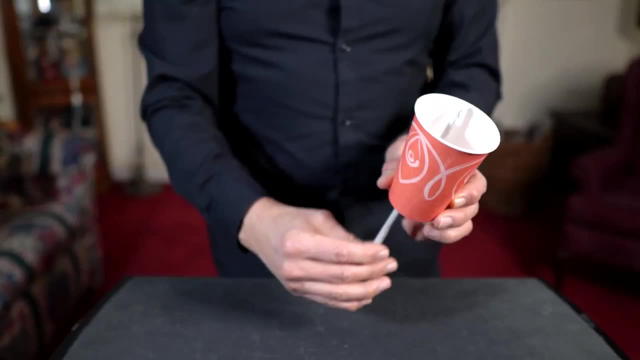 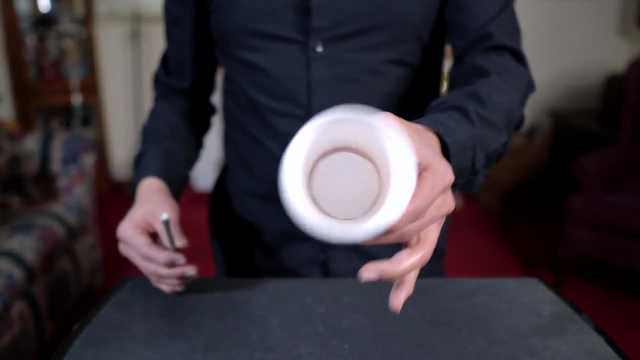 And you can show it from the different sides. Now, when you push your pencil through, you just kind of shake the flap and it goes flat. So you can briefly show the cup and show the pencil and you have a miracle. There you go. 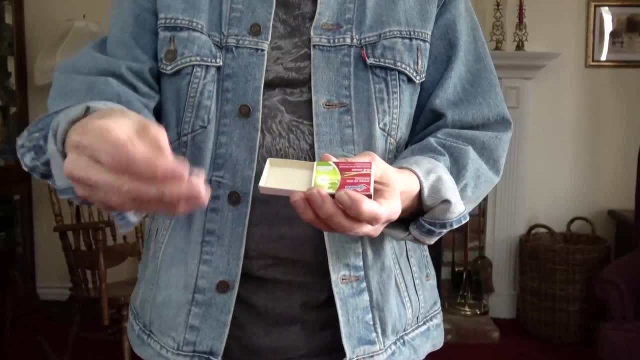 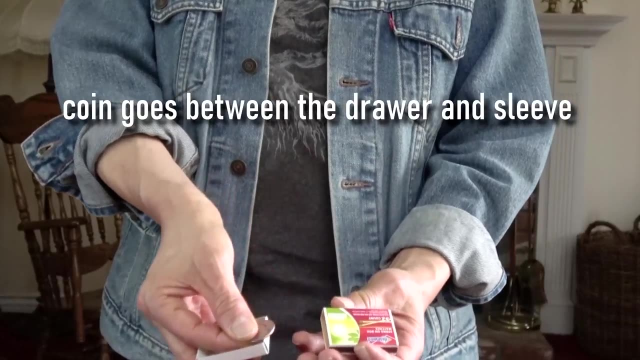 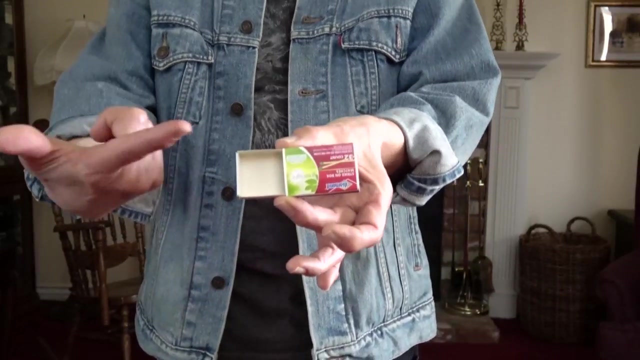 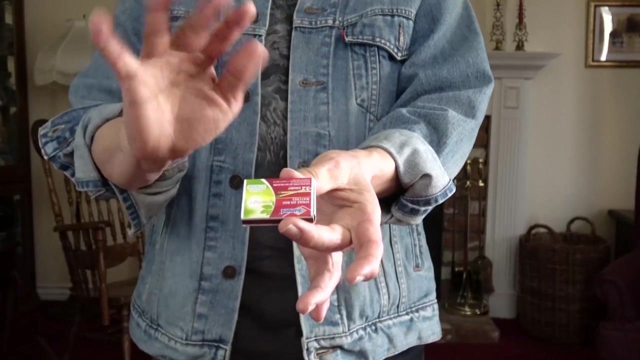 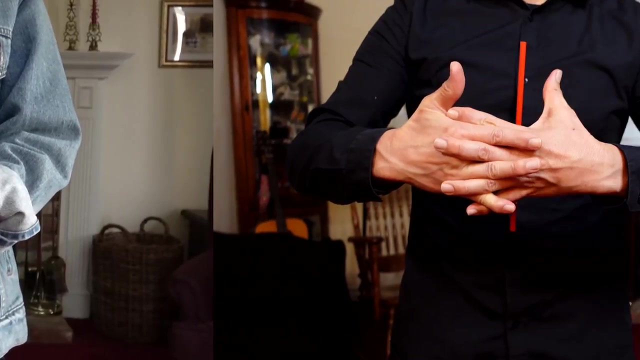 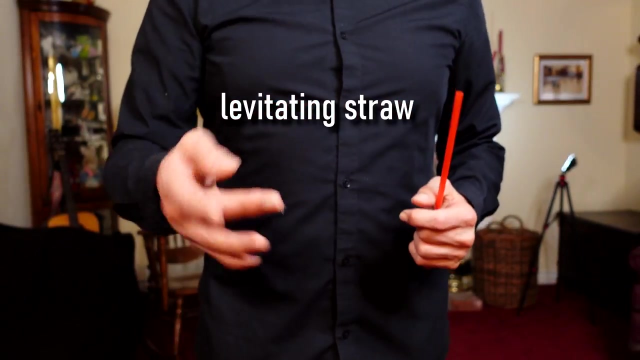 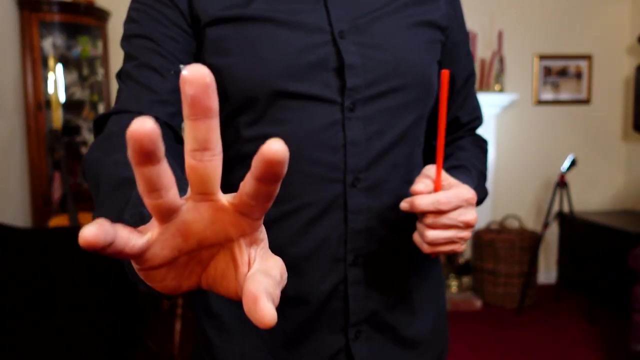 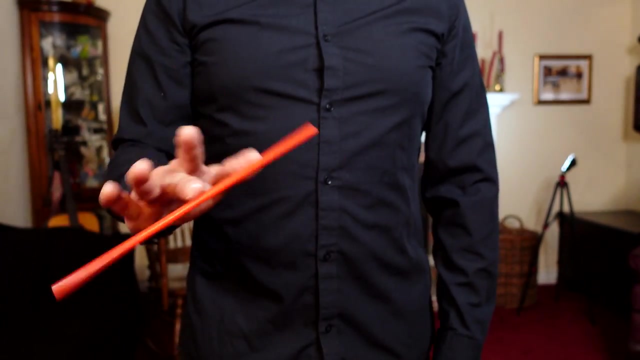 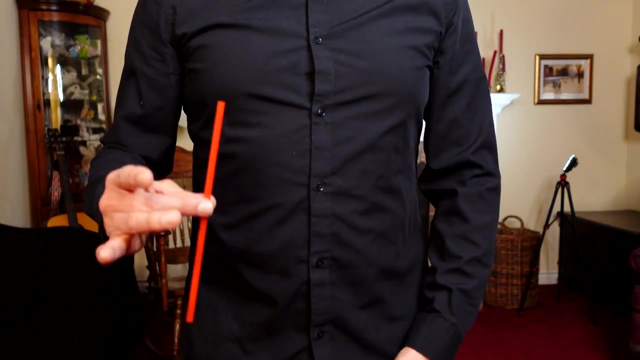 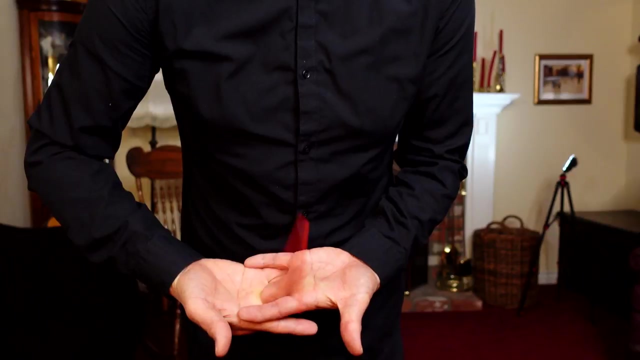 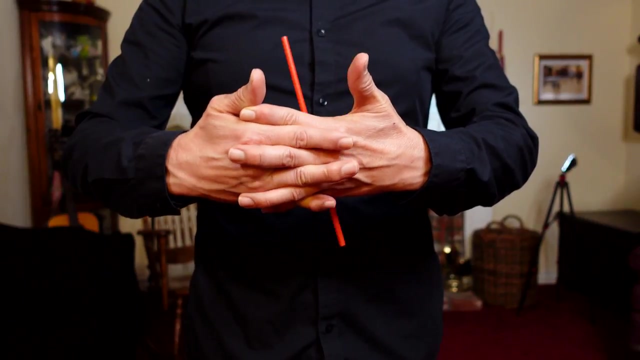 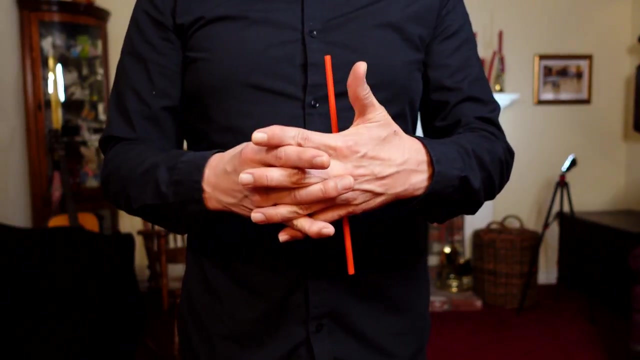 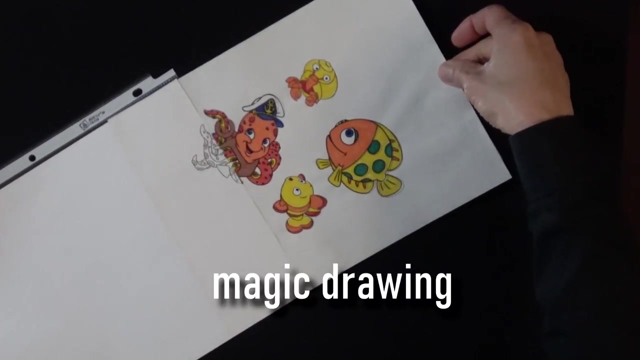 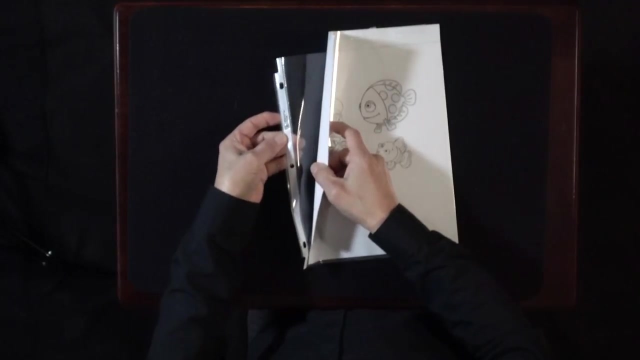 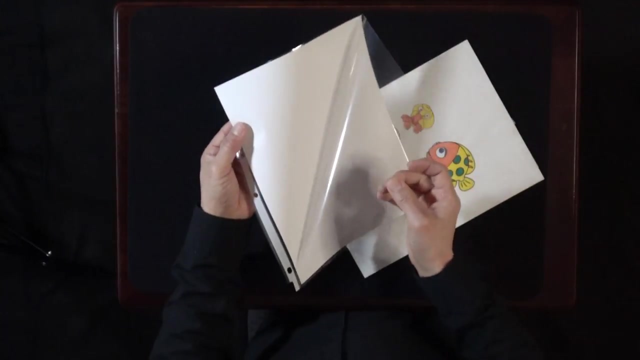 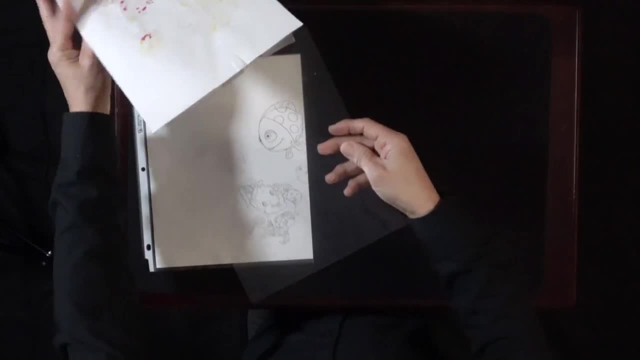 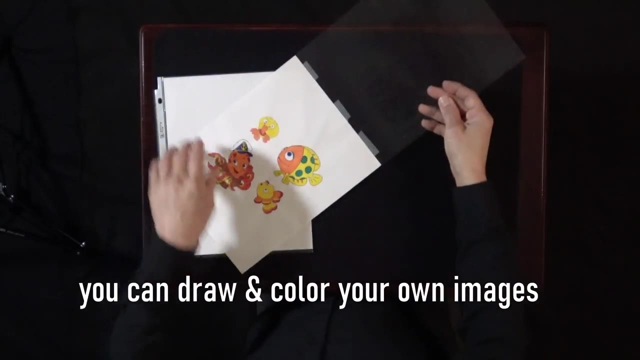 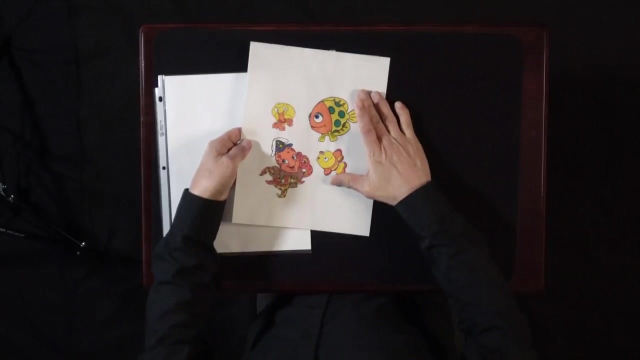 This is actually two layers here. The front is a transparency that has a black and white image And the back one is Color. So this goes over this And they have to align perfectly for the trick And then in order to perform the trick. 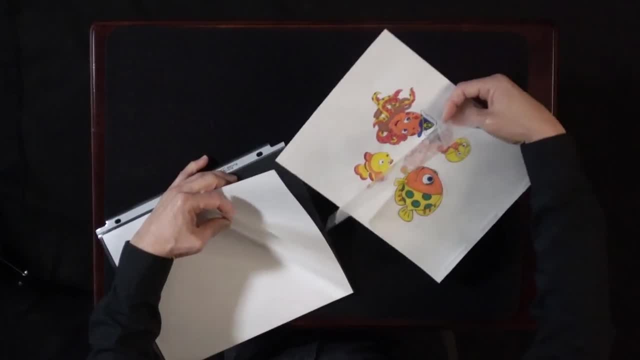 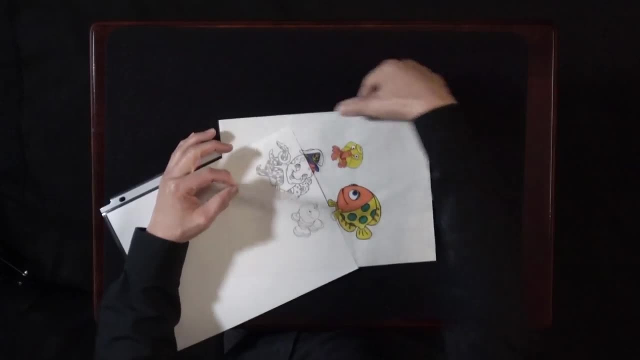 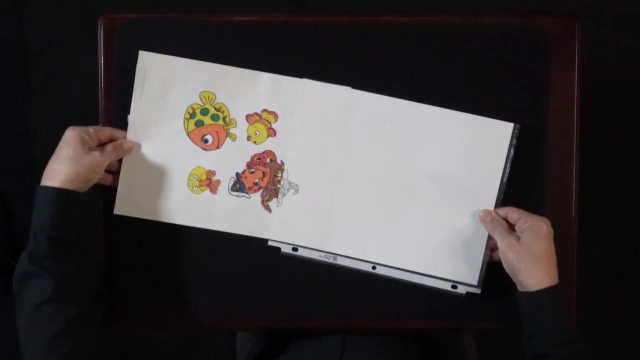 The color image goes underneath the white paper. Transparency: black and white goes over the top And from there, all you have to do is just Pull it out And you'll get this magic effect. And you'll get this magic effect. 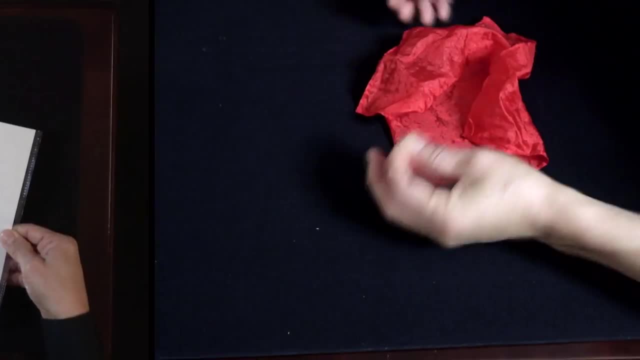 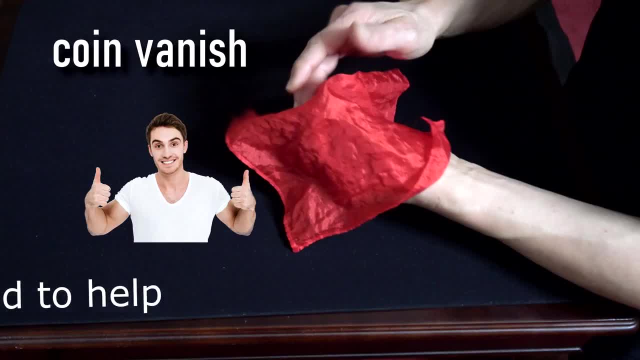 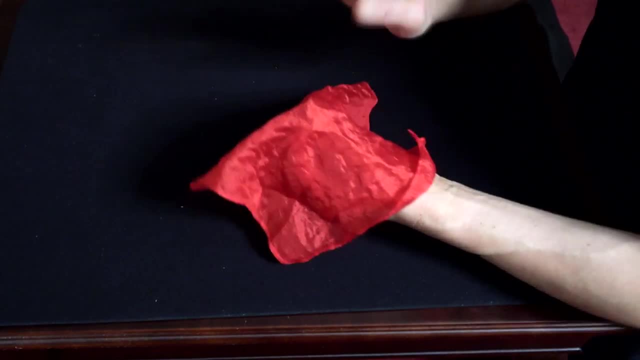 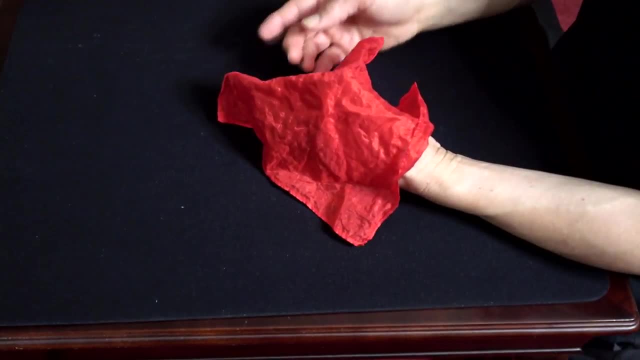 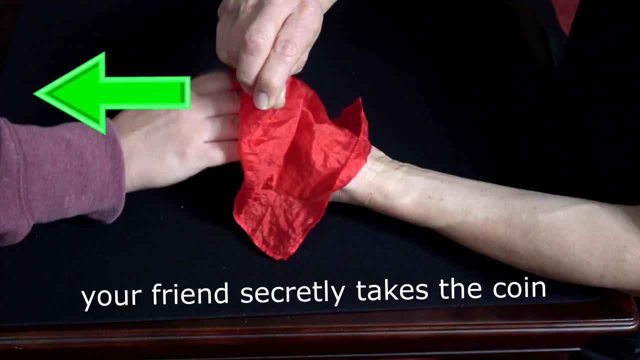 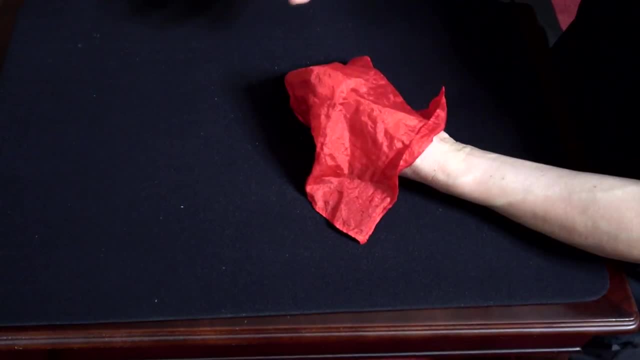 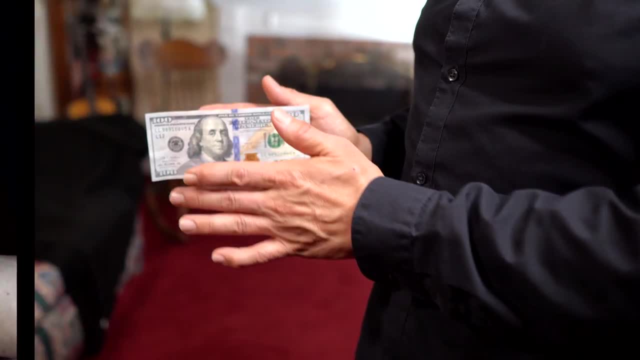 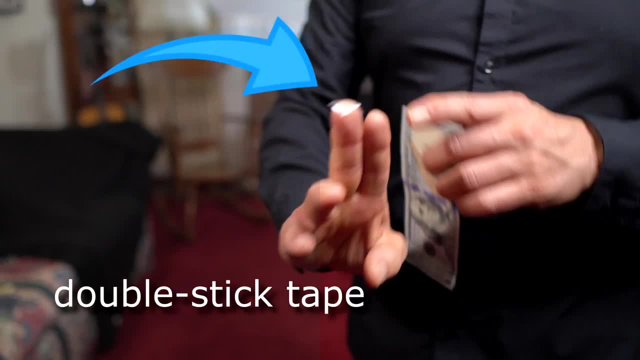 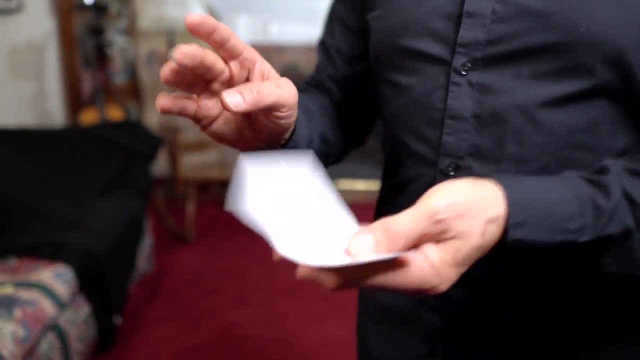 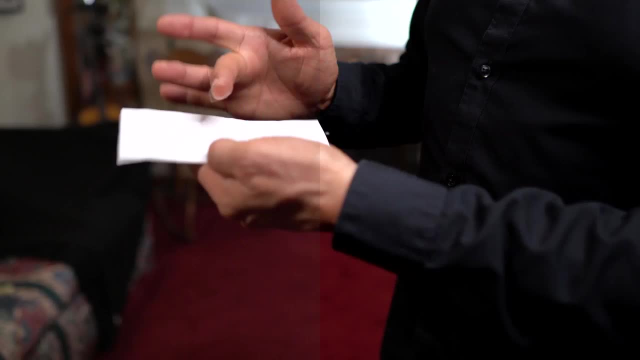 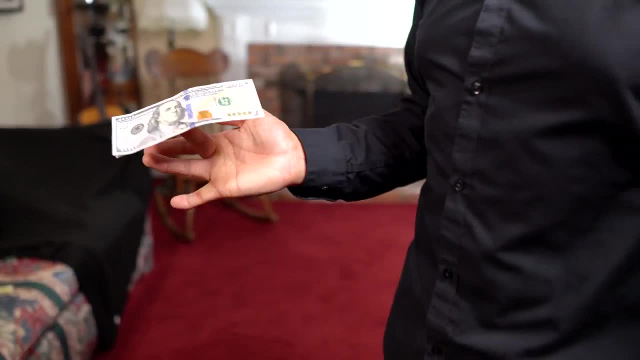 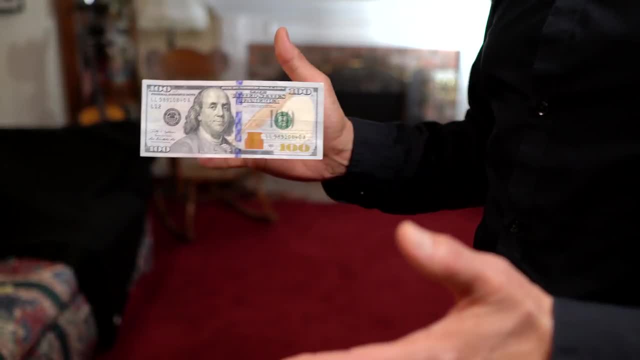 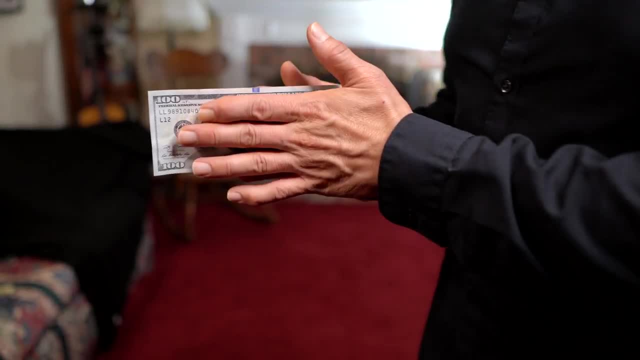 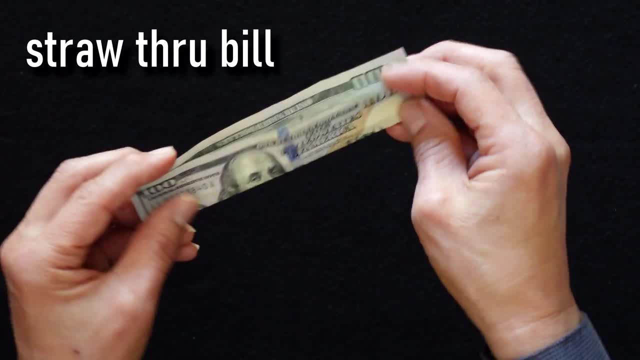 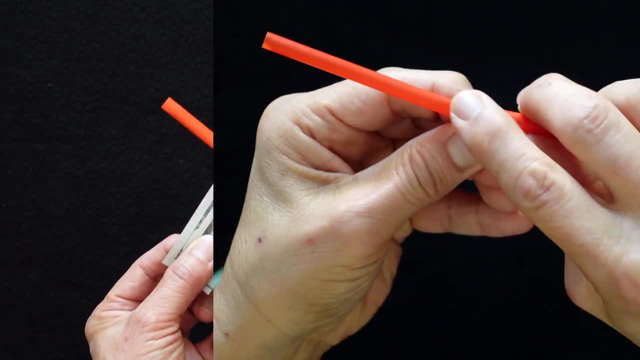 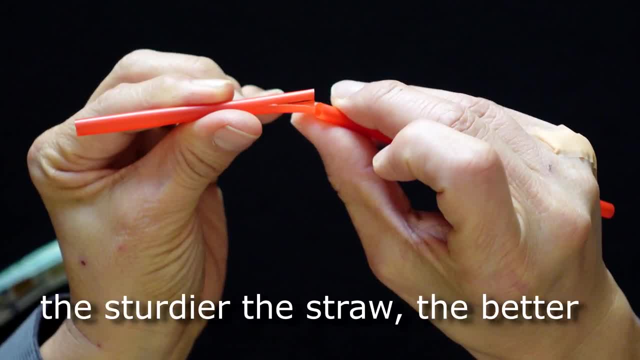 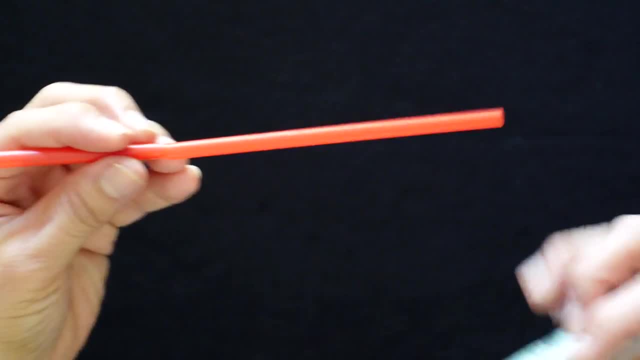 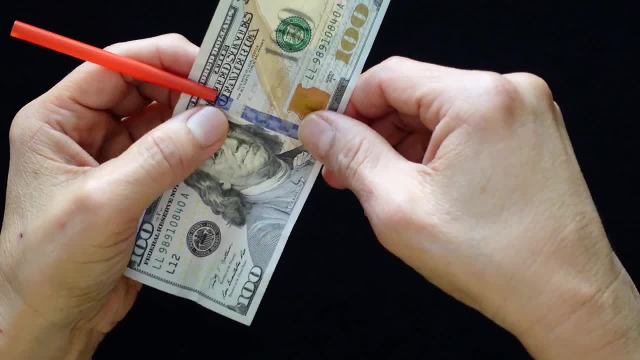 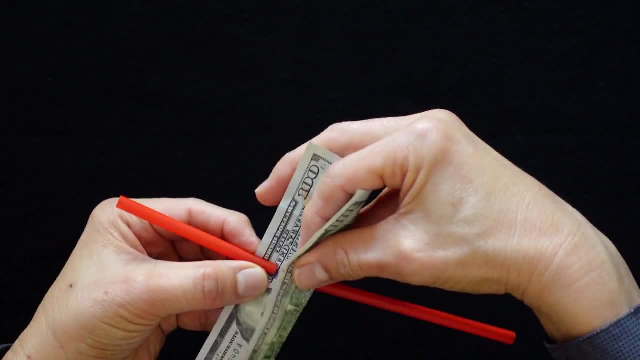 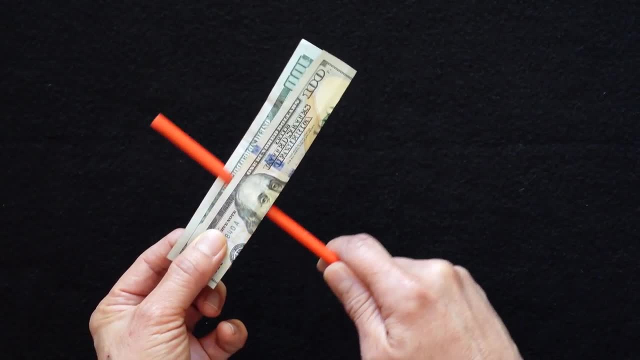 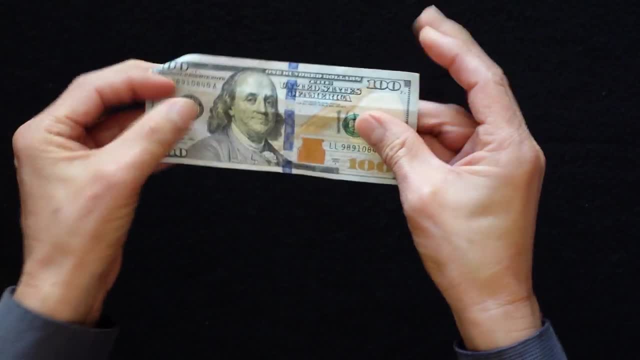